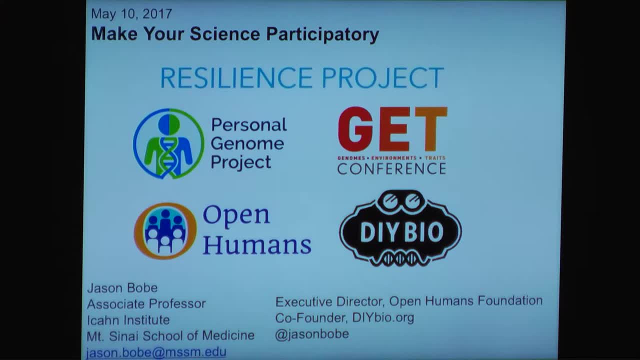 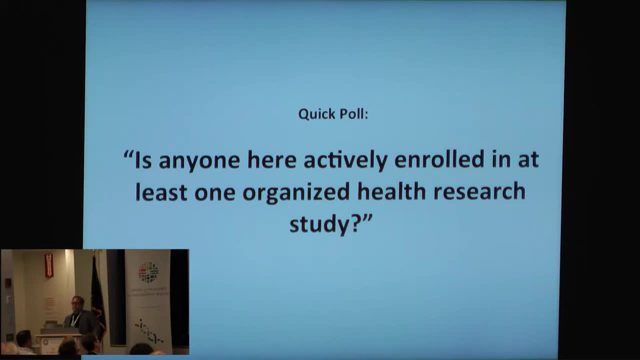 over the last ten years for this endeavor. But before I get started, one of the things that really interests me in my career is participation in science, And so I would just like to see in this crowd how many people are currently actively enrolled in at least one organized health research study where you've signed. 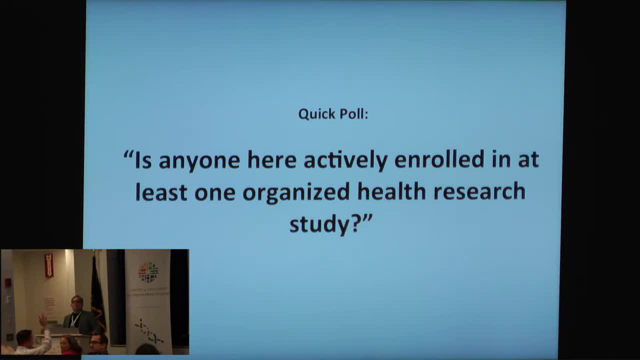 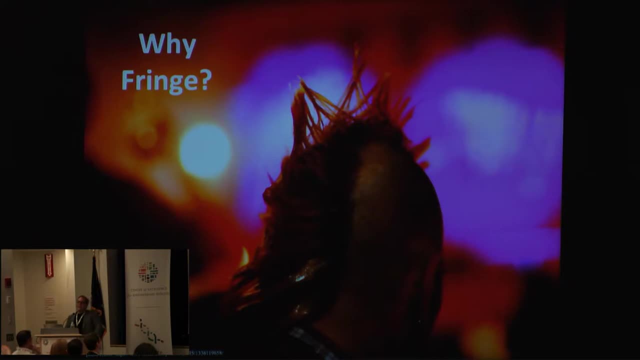 a consent form. Okay, so there's a couple hands, And this is really something that puzzles me. There's one in the back, also a late hand. That's good. So we're still pretty low, And I call this the participation paradox, If you ask people what they care about health. 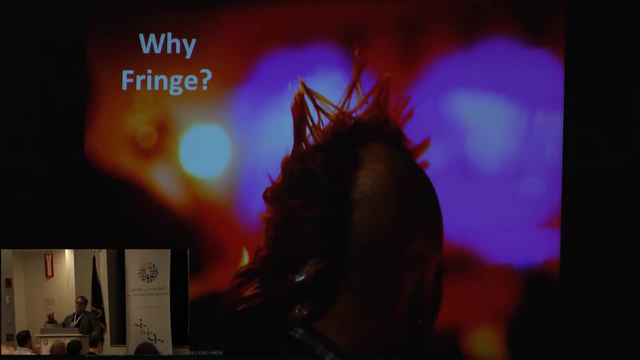 and healthcare are near the top, And who are the trusted professionals? Scientists, medical scientists are near the top of the stack. Marketers and lawyers and business leaders are near the bottom. Politicians are at the very bottom, And so if people care so much about health and healthcare, 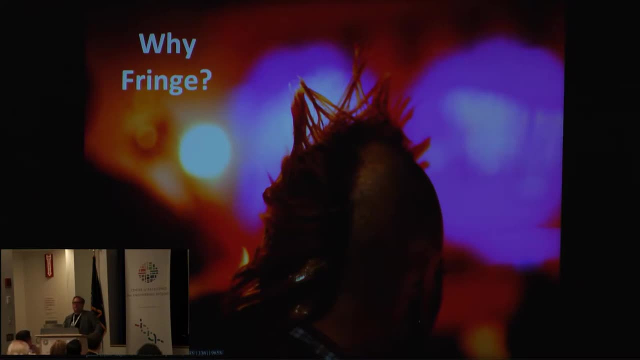 why don't people view research as a tool for solving the challenges that face their families and their communities? And I think that's a major problem in our society right now, And so maybe you can help me think about that and solve that. But also, we're starting to 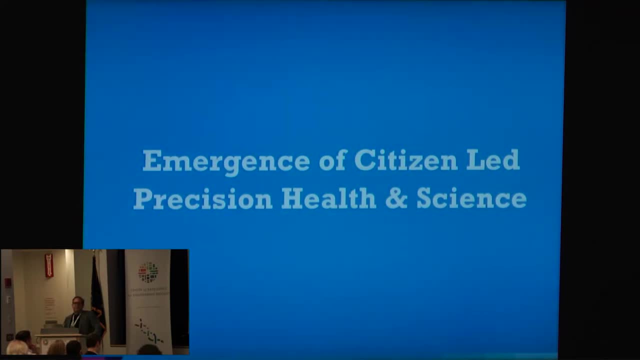 see a lot of people adopt research and scientific tools and practices on a really grassroots level. This is a really important movement that needs to be nurtured And this endeavor needs to figure out how it can relate to these individuals and these groups who are excited and passionate. 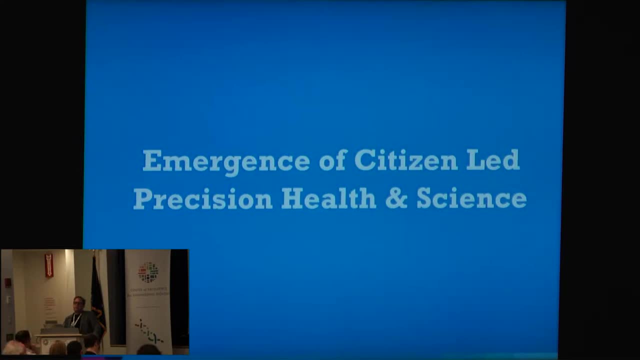 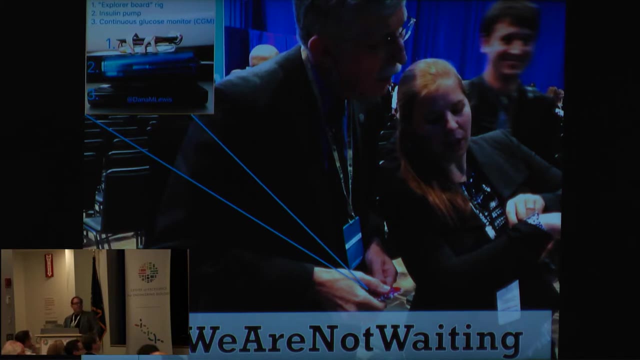 about how research can solve the challenges of our era, And so I just want to give you a couple examples of things that I think are really exciting, that you can go look up. That's breaking news. That sounds pretty interesting. actually Something about FBI, I'm not sure. 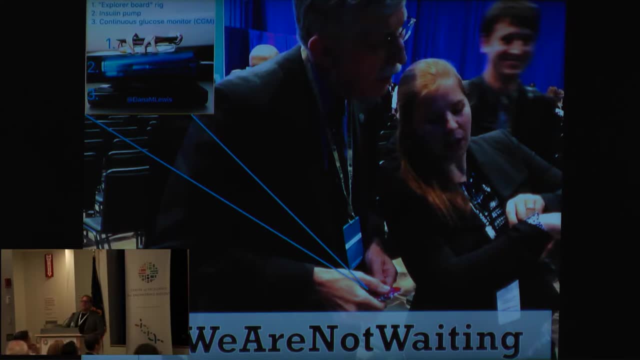 So this is Dana Lewis, and she runs an effort called OpenAPS under the hashtag WeAreNotWaiting, And this is sort of. I just want to bring raise this example of the ingenuity that exists out there of people who are really passionate, And so she's actually created an open source. 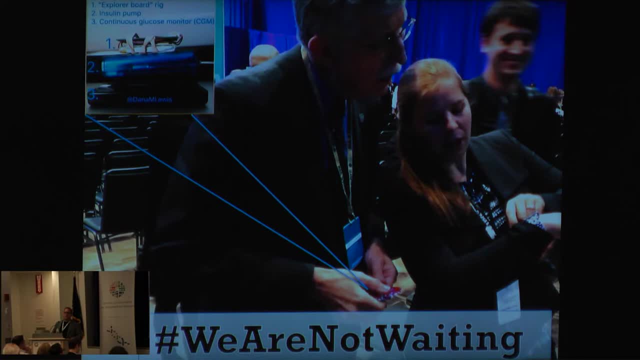 stack of hardware and related software for her insulin pump, because the medical device companies who were working on this only made the data available to the medical doctors and not to the individual patients, And there's a lot of reasons why that's a problem for 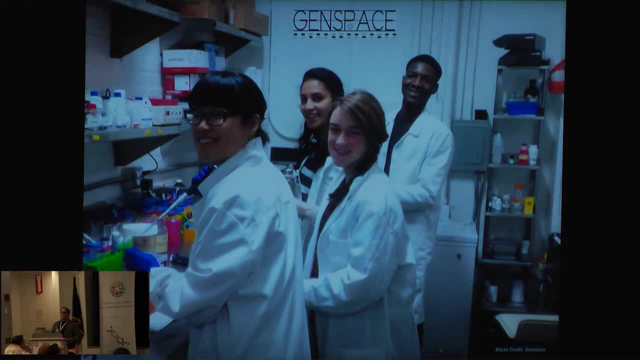 this community And then also a local community which I think you have heard from a few of these individuals. maybe met Ellen and Dan, who are here, and some other members, Genspace. So this is some new faces of people who are practicing science And there's just now a concept of community. 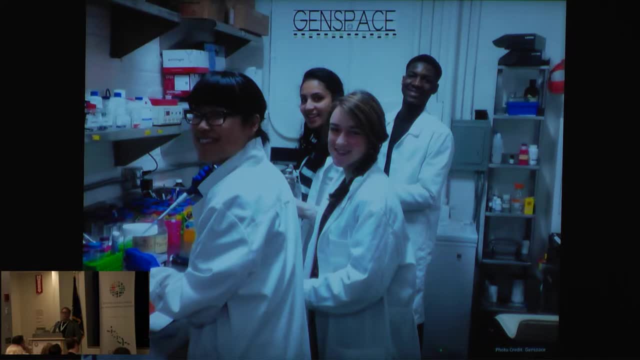 labs, And these are really all over the world And there are quite a few really great ones in the United States And Genspace is in Brooklyn And some scientists are actually partnering with them, like Chris Mason, who was here yesterday- I'm not sure if he's here right now- on the Medisub project. 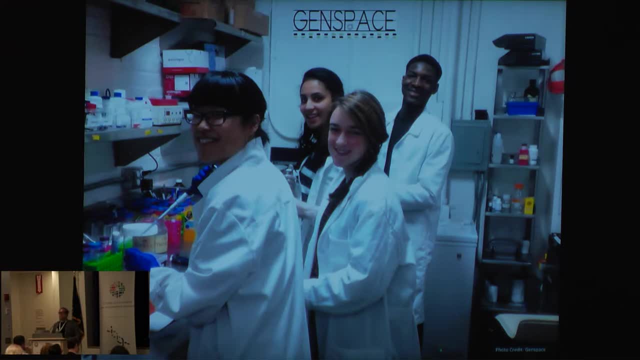 But basically some of the boring stuff that the postdocs would rather not do, of like doing PCRs and amplifications, of sort of outsourcing that to community lab, to be involved in projects where community members who are really excited may be way more excited to. 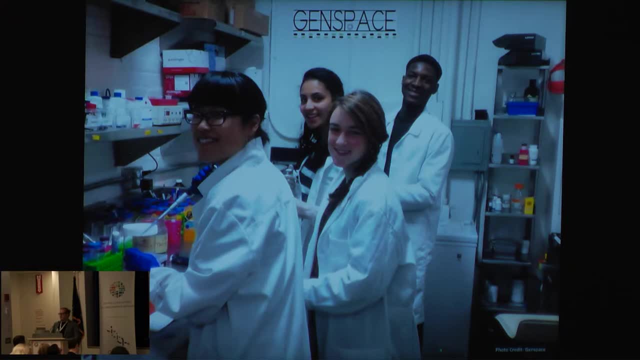 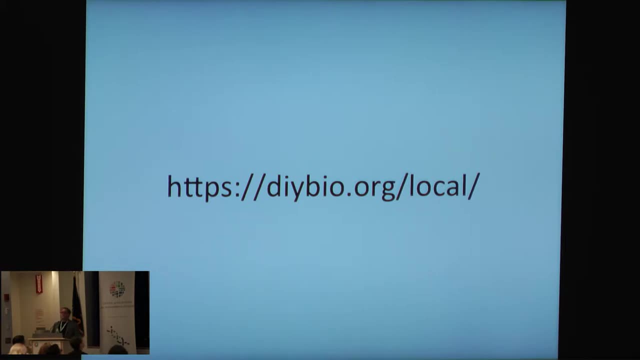 do a PCR than a postdoc, And I think there's a lot of really interesting opportunities there, And you can find more groups like this on this website. It's DIYBioorg slash local And maybe you can find some new collaborators and partners. 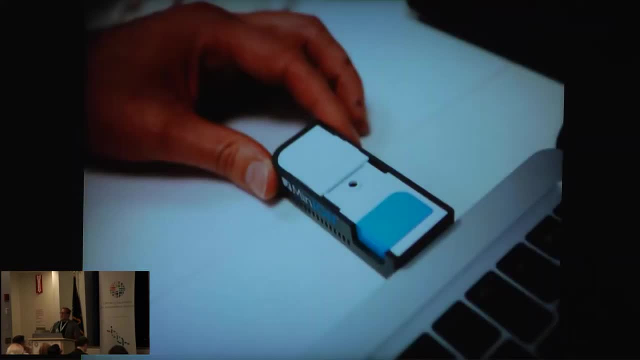 in the community to assist in your endeavor. And then also, of course we've heard about the drop in the cost of genome sequencing. But I think sort of more important than the $1,000 genome is a $1,000 genome sequencer. 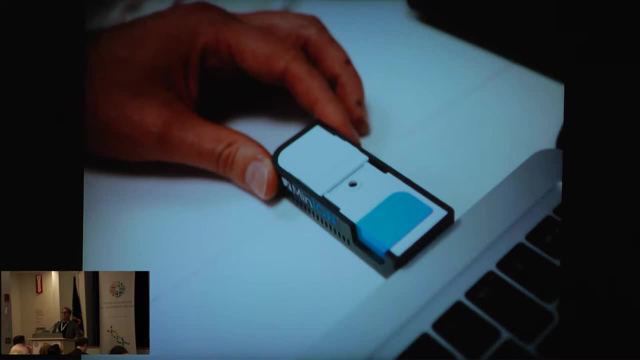 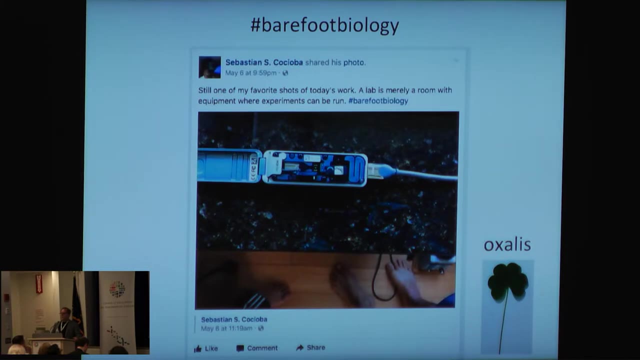 And we're starting to see the sort of fruits of the shift to individuals starting to do their own science projects. And so here in New York City there's actually a guy named Sebastian And I encourage you to go find him. You can find him on Facebook and follow him. 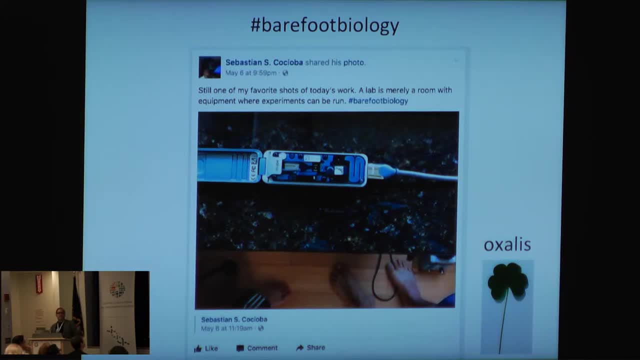 He's been posting several times a day now And he has one of these Minion sequencers And he's found this plant that grows like a weed, that you'll see it around New York. that looks a little bit like a clover oxalis. 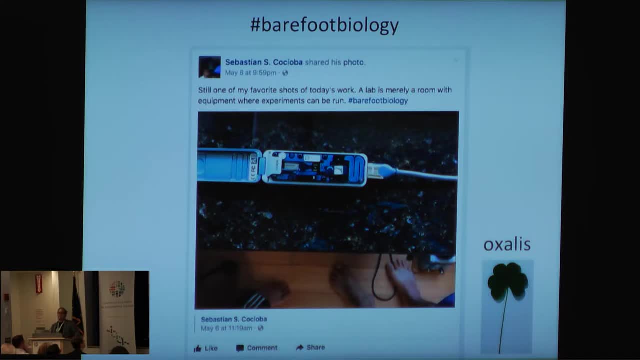 And he's been actually sequencing this genome from his New York City apartment using one of these Minions, And his hashtag is Barefoot Biology. You can actually see his bare feet here at the bottom from his kitchen, And I think this is a really important harbinger of where things are heading in the future. 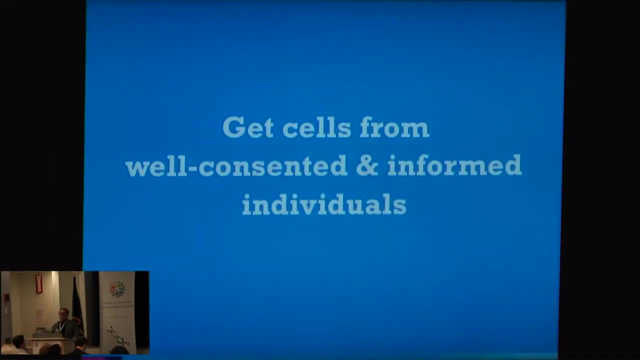 So back to sort of some of the opportunities that we have here for this endeavor. So, to the extent that those of you are working with human cells and that you want to actually share the work that you're doing and the genome sequence data and all of the other omics data, 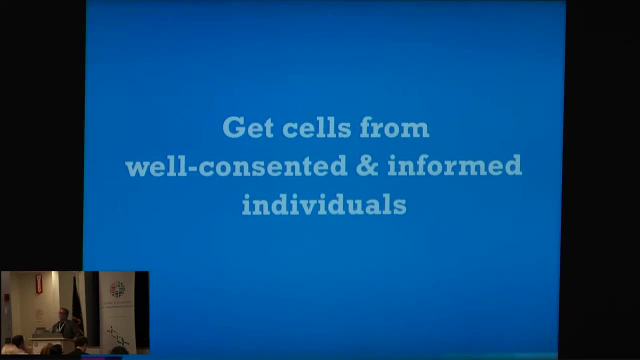 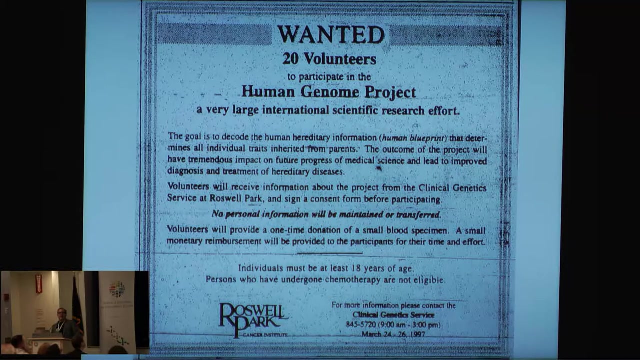 on these cells. I would really encourage you to find really well-consented cells and people who were those cells derived from. And so I don't know if any of you have ever seen this advertisement, but this is actually the original recruitment ad for the Human Genome Project. 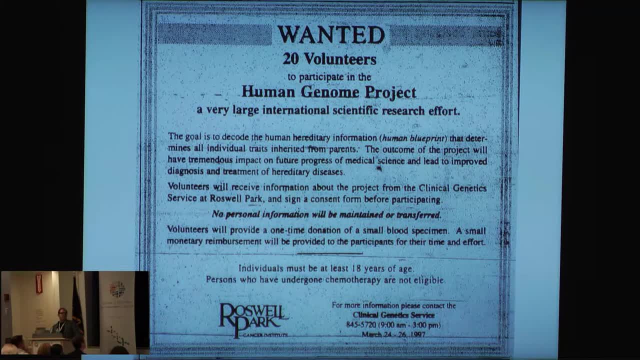 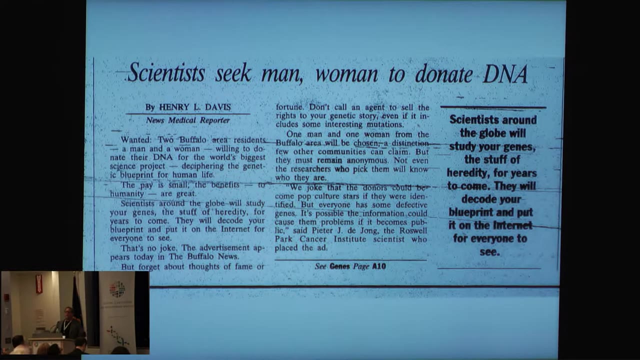 And so you can imagine that this endeavor is going to have some sort of recruitment advertisement, looking for people who are willing to donate their cells, sort of in a similar way. So if you read the accompanying article, scientists were seeking somebody to contribute to this. 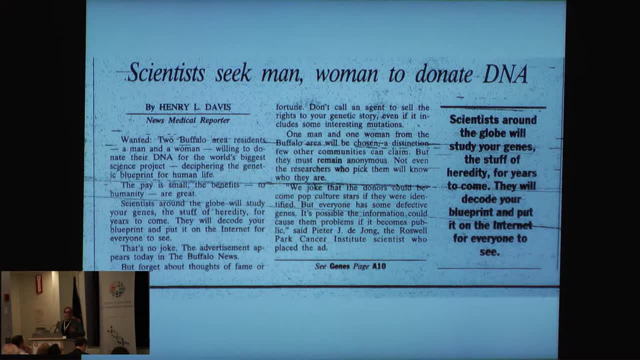 endeavor and it says in there. it says, look, we're going to put it on the internet for everybody to see, but don't worry, nobody's going to know who you are. And so it didn't exactly anticipate some of the challenges that were coming with identity. 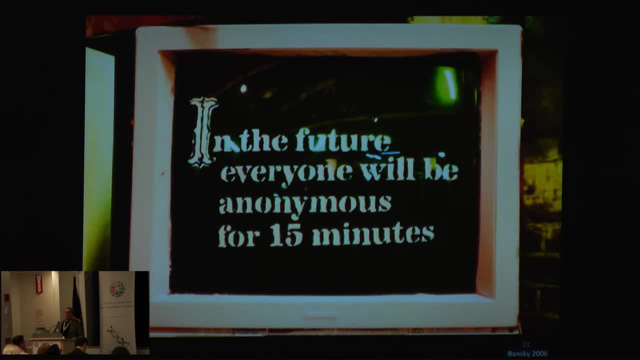 that Bansky sort of saw that was coming online around that time and people starting to understand: hey, there's a great interest in genealogy and people are just really ingenious. And so around the same time as Bansky also there was George Church who said: hey, you. 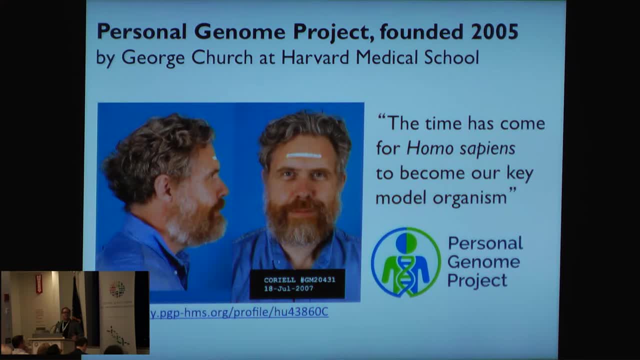 know this is a really it's time to make humans the key model organism to advance our understanding of human biology. And so you know that's what we're looking for. And he said: you know there's a couple challenges. 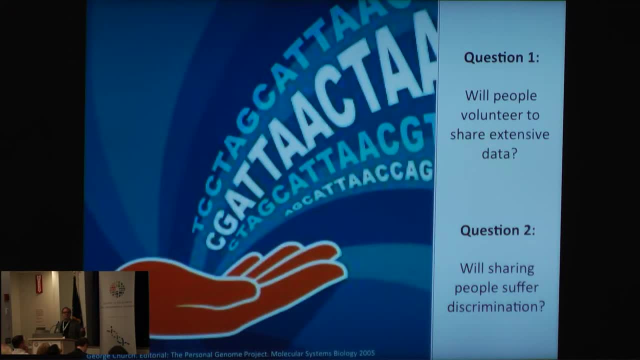 One is: it's unclear whether or not people will volunteer to share extensive data and if they do, will they be discriminated against? And that was really an open question in 2005 when he published this. You know this was pre-Gena, and then, of course, the Affordable Care Act and pre-existing conditions. 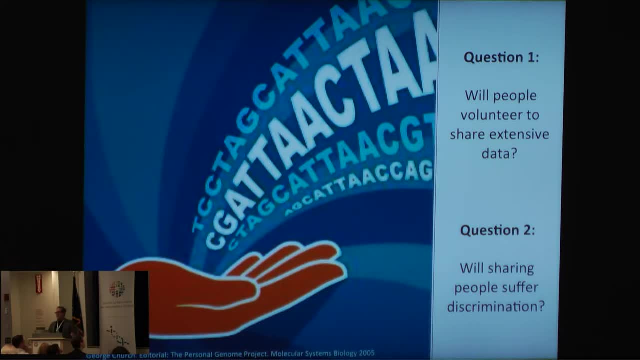 and we're still swirling around those issues today, And there's a lot of unique features of the PGP which I'm not going to go into them, but one that's really important is that it's participatory and it's about being informed. 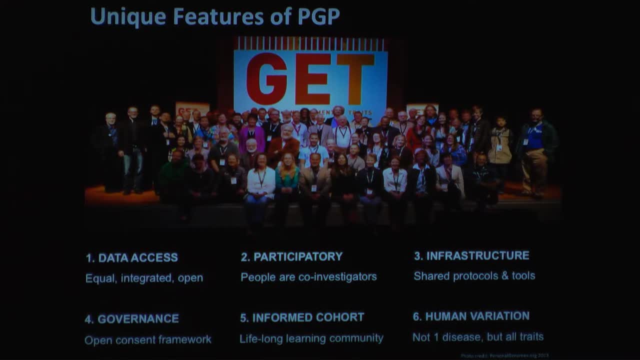 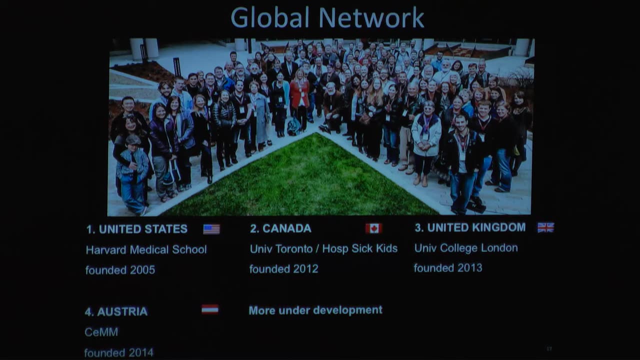 and being a learning community, And it's very different than a lot of sort of human subjects research that maybe you're familiar with, And there's also a global network and growing And people. one of the things that we learned from the early days is that, by designing a 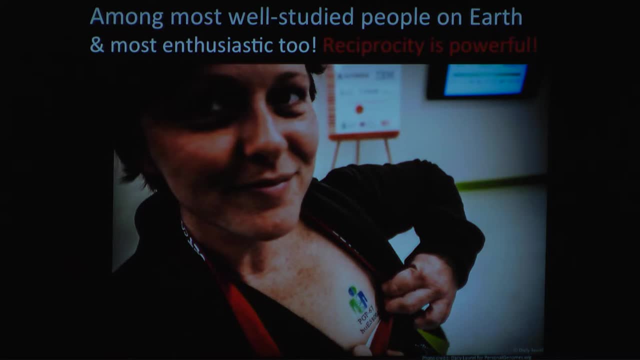 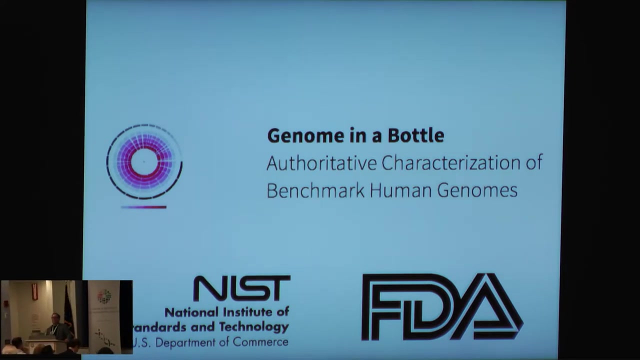 governance structure where that treats people, individuals as people, and where there's reciprocity. it's a really powerful force in forming relationships with people that you want to work with over a long period of time. And so This group- Mark Salitz here from NIST and the FDA- went around the world reviewing consent. 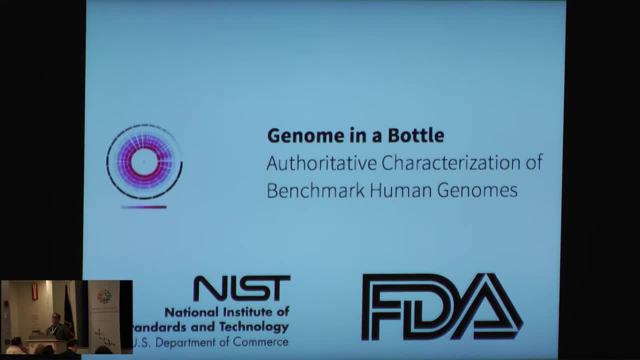 forms and saying: look, we want to develop genome in a bottle, where we literally are going to be selling somebody's DNA as a standard reference sequence so that clinical laboratories around the world can calibrate their instruments for the benefit of mankind, And we want to sequence this DNA on every platform and put it on the web so people can. 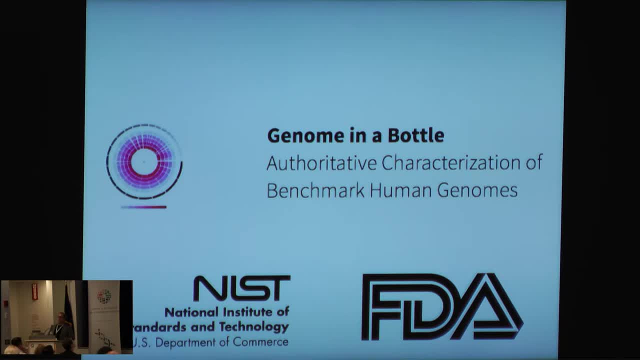 calibrate their instruments and, over time, have this really valuable resource. So That's the kind of thing we've done, And if a patient shares a profile of something that they don't know and they're going to have this service, that gives them the opportunity to say: look, it's one of the things I did. 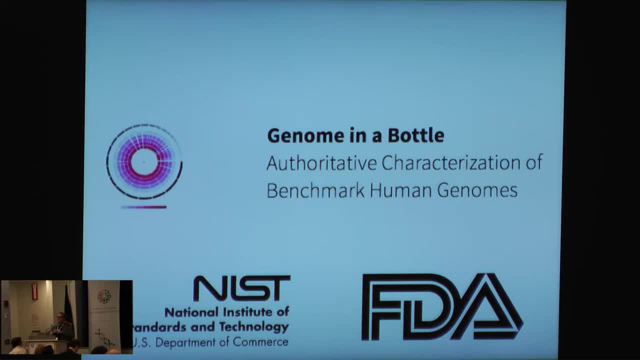 while I was here, I did this in an experiment. This is what I did, And then they're going to have a picture And if it's there, it's going to be, like you know, an exact copy. They're going to be able to sell their DNA. 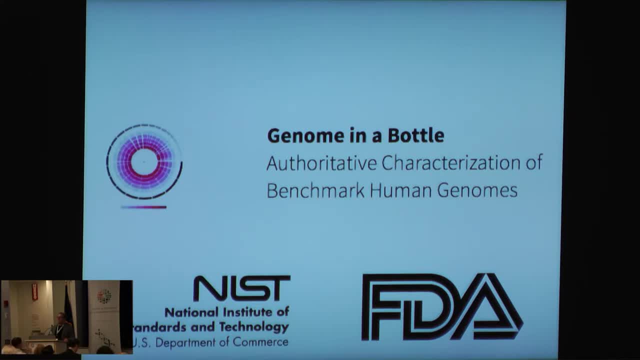 They're going to be able to get the DNA to the research center, But if it's a really successful sample, it will be a great source of time And I think that, like we said, We want to do it at a much deeper level than what we are doing. 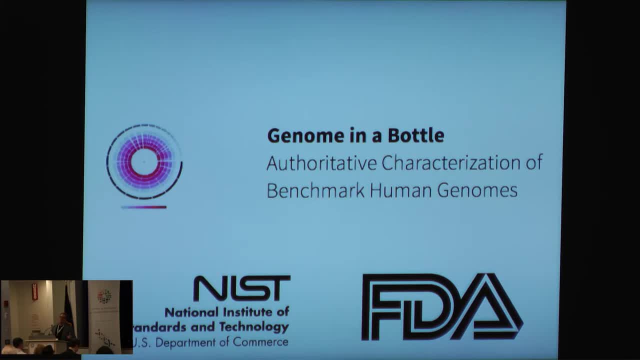 That's why the questions I asked about the Harvard Genome Project. we had an opportunity of the opposite of what happened to Henrietta Lacks, who's also in the news with the new movie it was. these are people who voluntarily said, yes, I accept these risks. I think this is important. 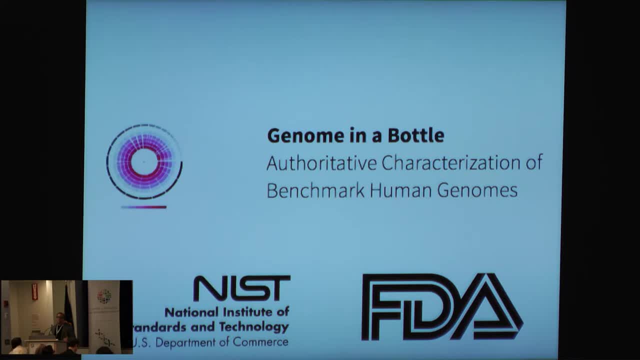 and I want to. I want to help support this effort, which is a very different circumstance from somebody who wasn't involved in those decisions and it came as a surprise. so you know, if you choose your own adventure, but I would encourage you to to choose wisely and so quickly just a few. 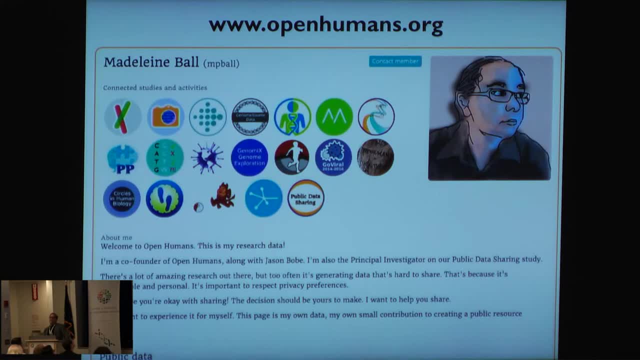 other things. I would just like to say: go check out open humans and this idea of people being excited about science and building a longitudinal integrated research profile from those research studies who actually allow them to have access to the data and and accumulate it over time. I think 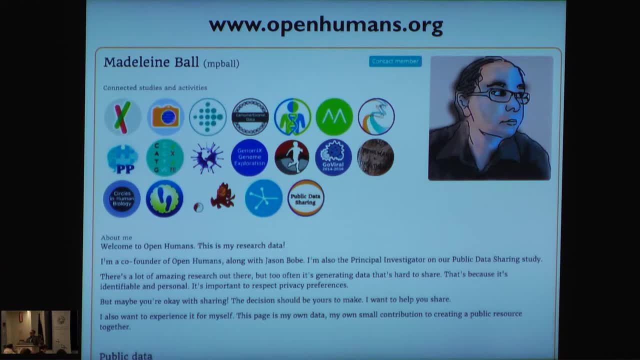 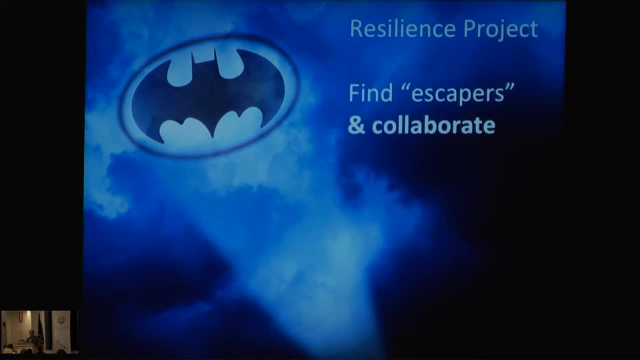 there might be an interesting model for some of the efforts in this in this consortium. and then also finally, I just want to say that I'm looking for individuals in in my most recent work in the resilience project for people who are really exceptional, who medical textbooks say they should. 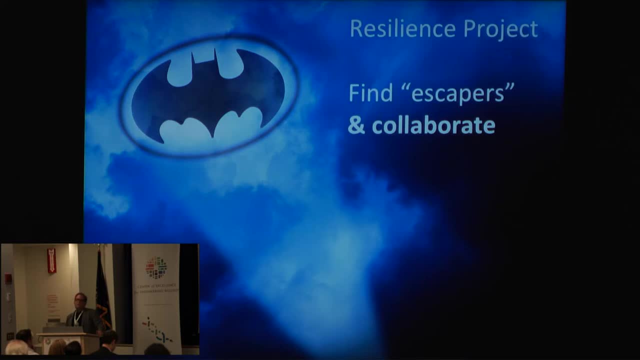 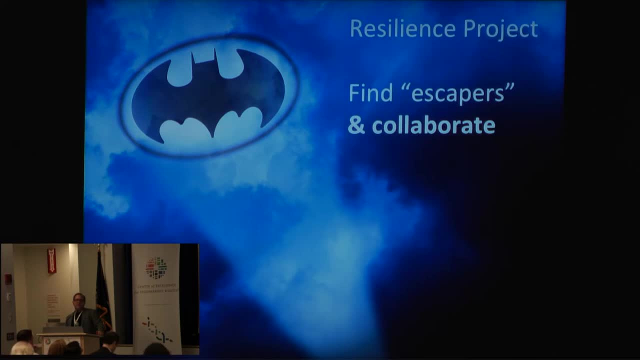 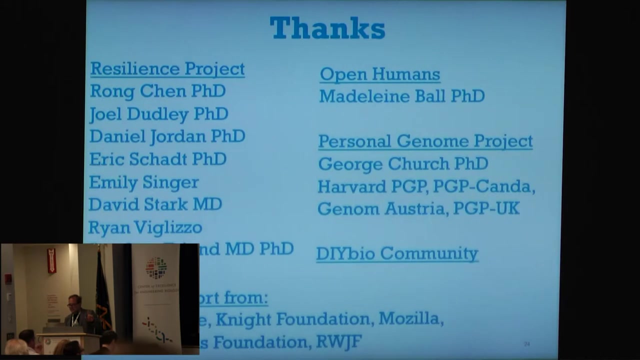 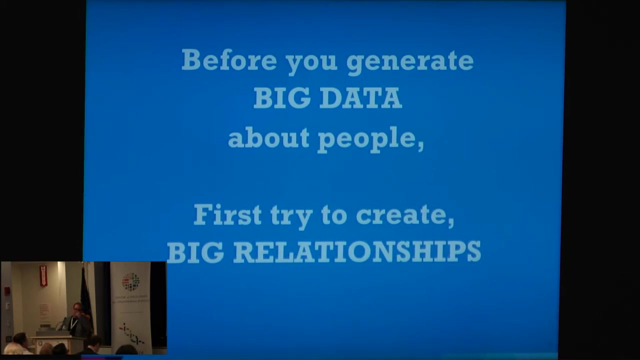 to explore and to, to, to go find, to actually recruit, to use their cells for, for research like this, and I'll stop there and take questions. thank you for having me. oh, I forgot, I forgot there's one. can I just add one thing? that was I ended too early. I want to say, I want to encourage you that 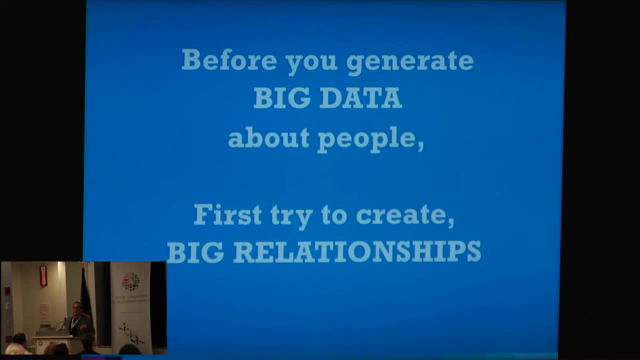 for, for those of you who are really excited about the possibilities of big data is to first try to create big relationships, and and for those who are really interested in why that's important, I'd be happy to tell you some some recent experiences that I've had where we've had 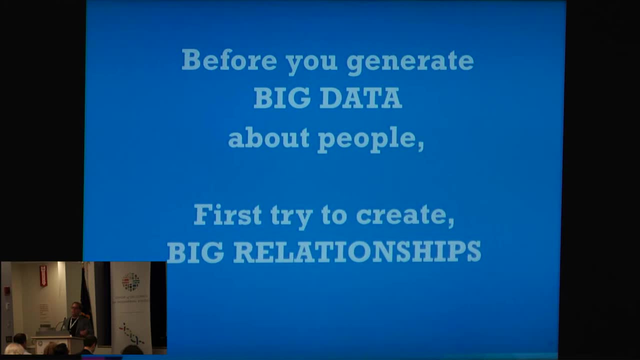 the big data but not the big relationships, and and our opportunity to do real science dried up. I wondered if you could say you sort of alluded to it. I wondered if you could say a little bit more about the idea of consenting people when the land's you know. 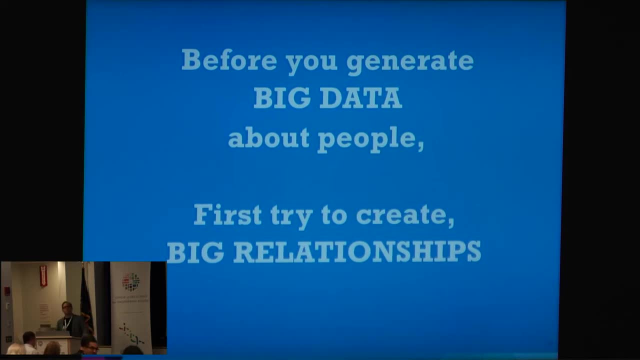 the landscape's changing. I mean, obviously there's um the fact that Gina doesn't cover long-term disability or life insurance, but also with the recent bill, there's this notion that wellness programs will allow people and end around Gina, and so does that trouble you? because it's obviously less likely to make people want to consent. and the landscape shifting. 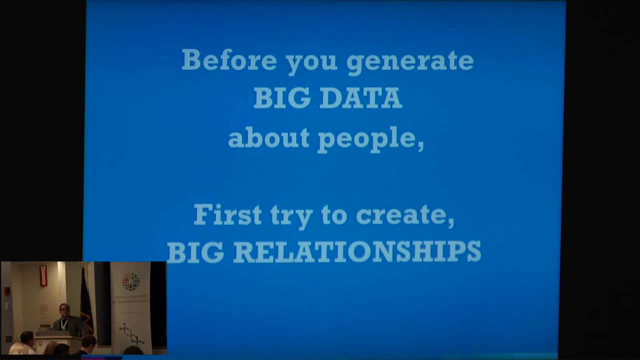 right. so I think this is another important reason to to organize your governance in a way that has big relationships and that you can actually go back and re-contact individuals. and there are more reasons than uh, there are more reasons than one why re-contact is important. you know a lot of. 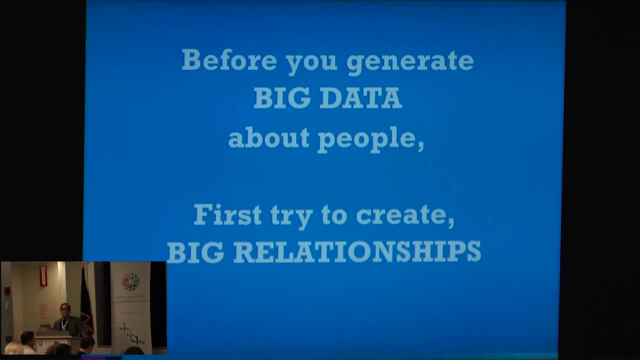 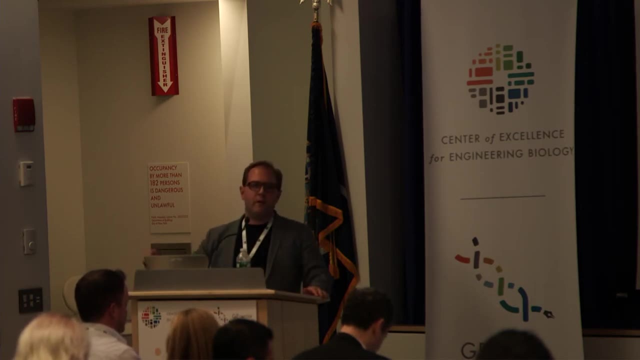 human subject research, sort of on purpose, creates memory holes where, like you, are not able to re-contact individual. and they are a number and you get. you know it's very transactional, it's like fill out a questionnaire and give a tube of blood and then we'll never talk to you again. 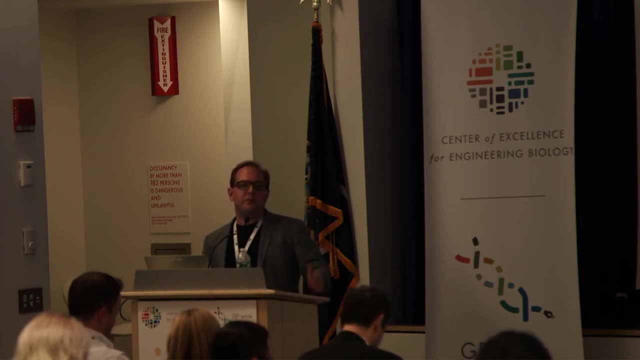 and there are a lot of reasons why you might want to be able to go back to people, not just to advance the science, but also to check in about changing circumstances in the world and whether or not somebody is still interested and invested in continuing to work with you or or on on whatever particular project. so I think there's a lot of reasons to sort of. 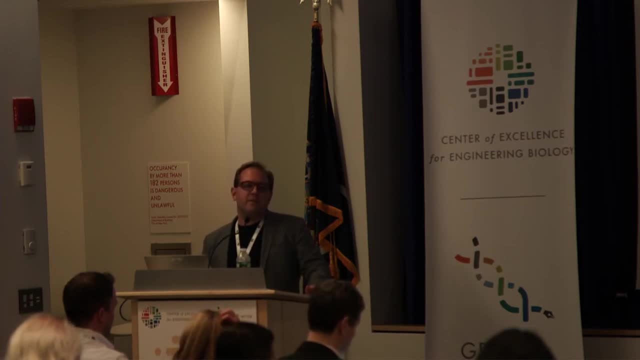 reorganize the biomedical research enterprise towards one that really values big relationships as much as it does big data? yeah, but did you does? does it make you worry, then, that the trend will be too for people to watch towards wanting anonymized deposition and not relationship building because of these things? 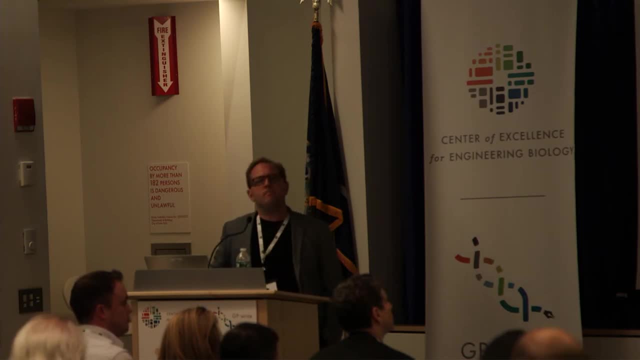 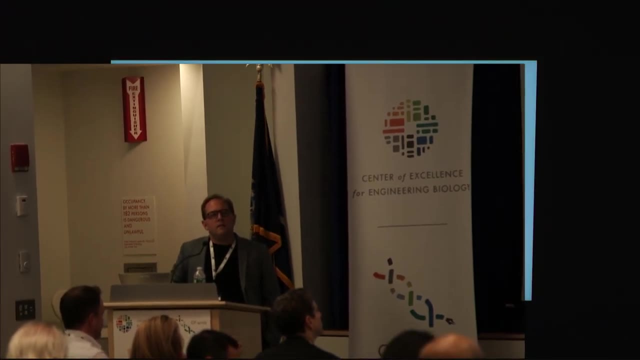 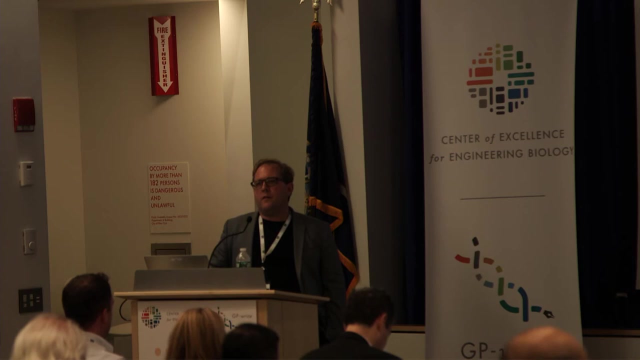 and actually it's. it's multiple steps back, because people fear and they say, I'll give it as long as there's no connection back to me, because a third party might abuse that, and that third party might be the government or the state. uh well, I do think that, um, that, uh, there is a relationship between 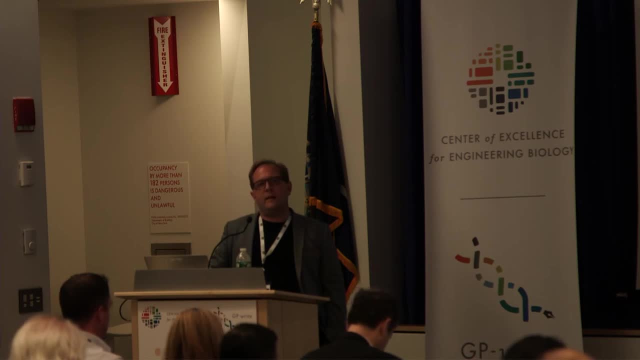 the, the protections that we afford people in our society and their willingness to take on risks in a research environment where, by definition, currently there can be no personal benefit and so there can only be risk. while that being said, I think there is a substantial number of people who are there are there are definitely certainly people who are more secure than other. 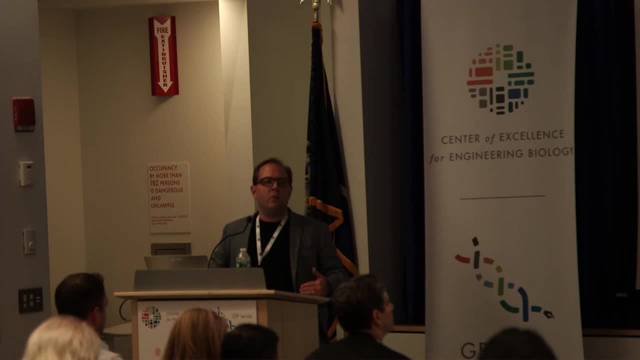 people and willing to take on more risk, and I think it's important to for people to be able to assess their own circumstances and make that decision. yes, there's a lot of people here from many different countries and, um, the kind of consent procedure that you're talking about is really about consent in the us right. so in your work in other countries, 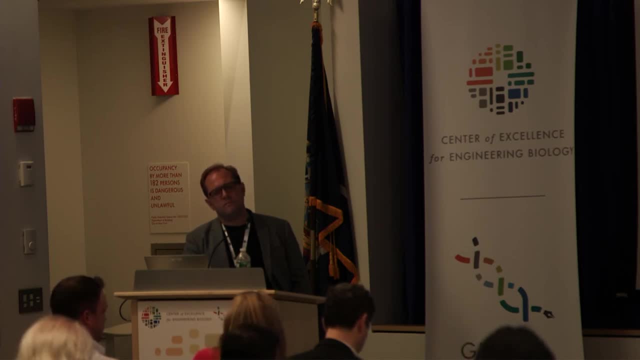 with the projects that you've been involved with. how have you found the local laws or the cultural conditions different, uh, in terms of the consent process and how it works? yeah, um, so you know, uh, uh, I, there are certainly a lot of differences around the world and in terms of 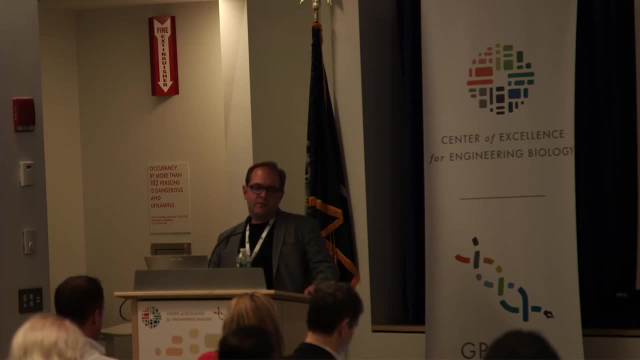 the in the early stage in the personal genome project at least, which intended to be, was intended to be global. uh, we decided to approach it through uh partnerships with local people who would understand local customs laws and not try to do that from Boston and understand what is appropriate.